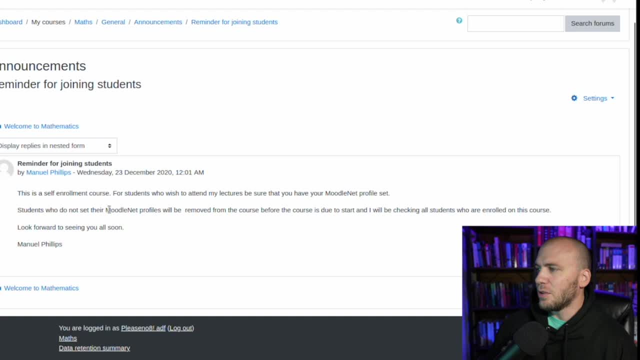 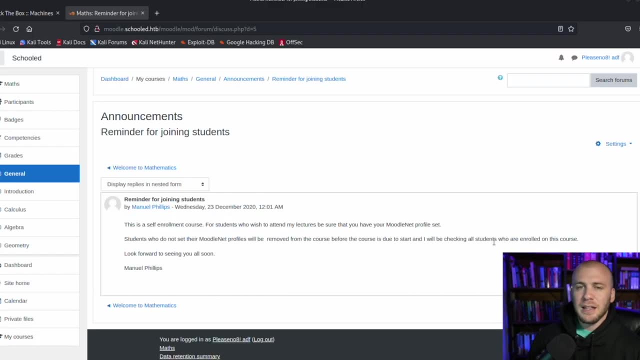 the course and that doesn't really matter, but it says that you're going to be removed from the course. they're going to be manually checking something right here. If you ever see something like this inside of a capture the flag, then this is going to be a cue that there's probably some 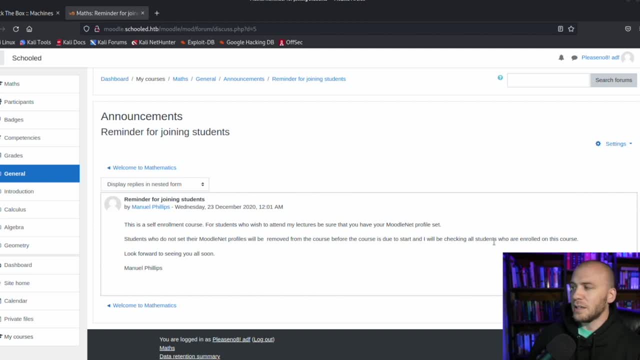 kind of automatic process running in the back end that is going to be checking this. so you know that somehow you need to be exploiting that. I've seen this with FTP before, where I got a file off an FTP server and it said it was going to be checking all the files that were uploaded to it, which meant 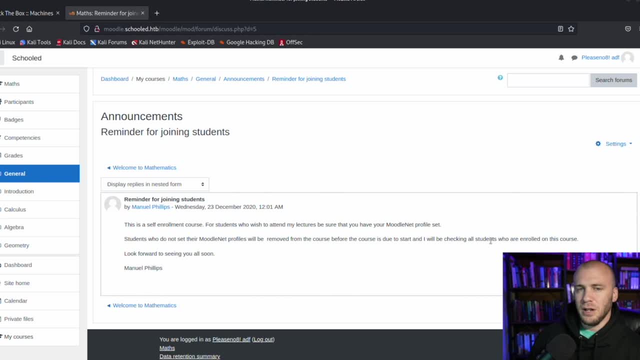 we had to upload a document that then was executed on the back end. So this in a capture the flag is going to tell you that some something's running on the back end and we need to exploit it. and we're told that it's going to be in the profiles, so we can come to the profile right here and then 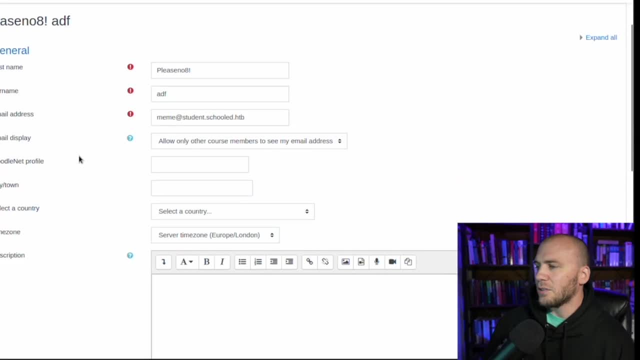 we're going to edit the profile and if you're looking for a cross-site scripting, there's a lot of different ways to look for them. but if you're going to come across one in a capture the flag, you can just come in here and you can do something simple like put in a bold and then something, or 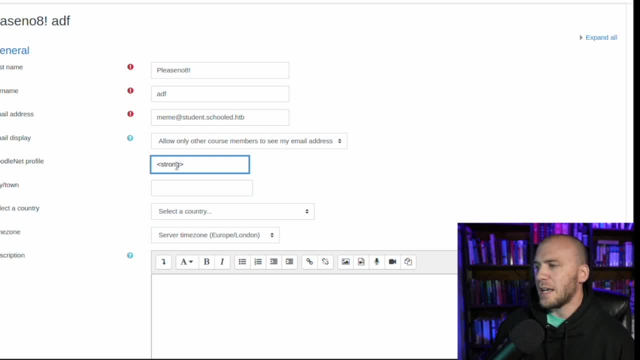 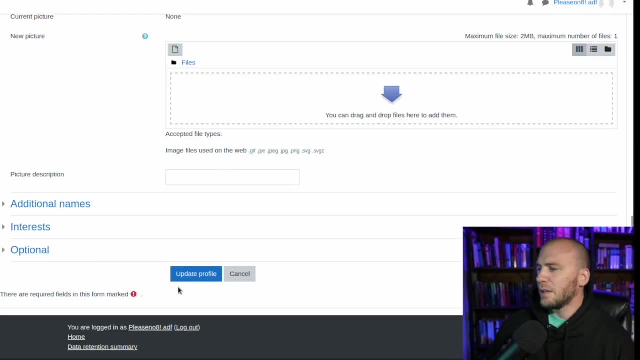 you can put in an emphasis, or you can put in strong or some kind of tag like this, and what will happen is it will execute this. So let's go ahead and close this off and then, if we hit update, it should emphasize for this, for us, which is basically strong, is just going to make it bold. 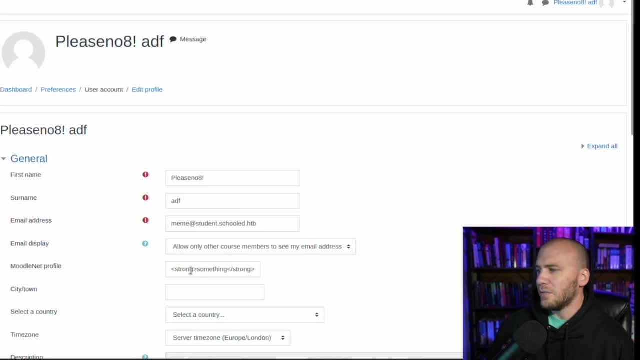 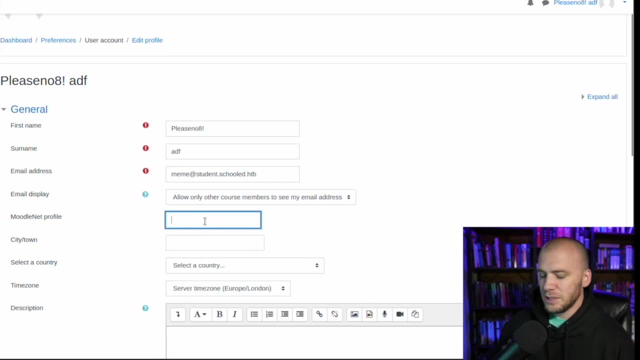 an easier way to do that would just be with the b instead of the strong, but we have this right here, so we know that it's executing html. I'm going to go ahead and type out the page name and then this is going to be the payload that we would need for this, and if you wanted to check this, you. 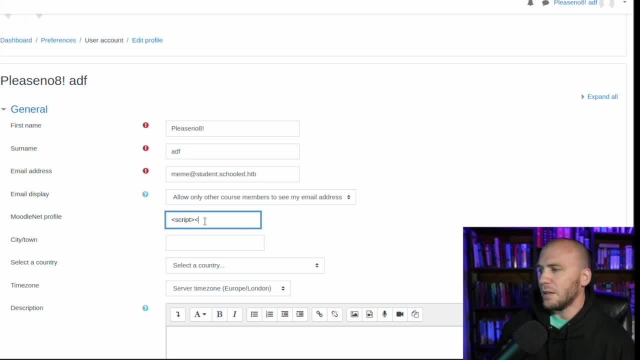 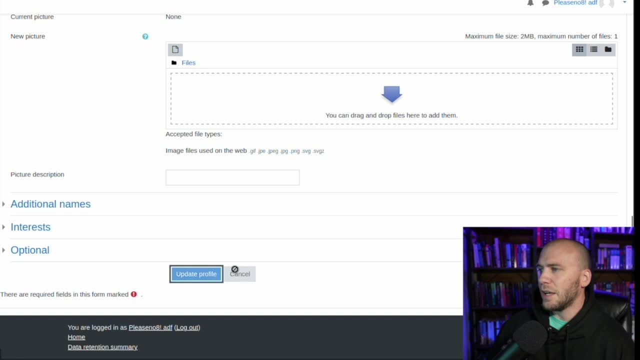 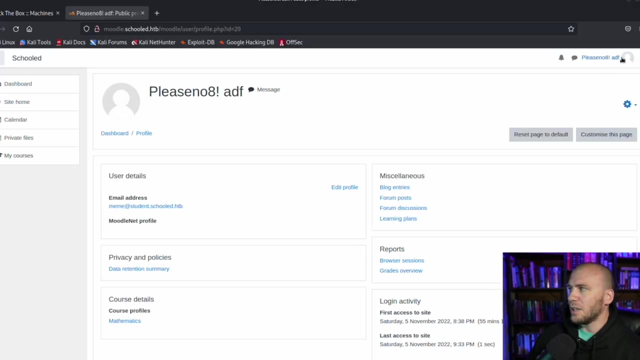 could actually go script like this and then a script tag, and then we can put our alert in here and then we could update the profile and it should pop in cross-site scripting for us. and we have it right here. so we know that cross-site scripting works. but I want to show you how to actually steal. 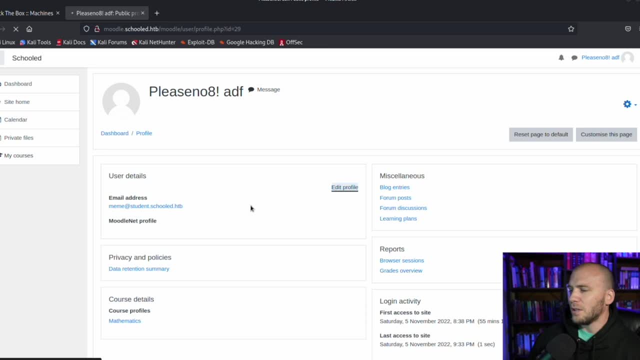 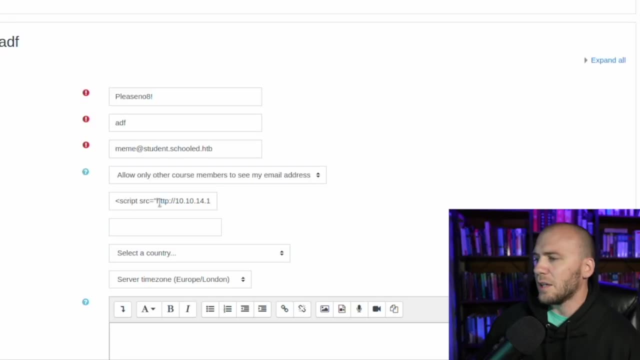 the cookie and then my username will change up here. so if we come in here, what we will? I'm going to type it out and then I'll walk you through what is going on here on. okay, so we have our script tag and we're just going to put the source to the script as our ip. 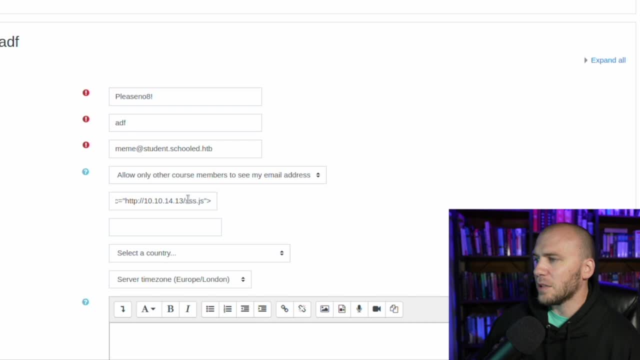 address which you can see. i have my ip address right here from hack the box and then we're going to have it go out and grab a file for us right here, cross-site scriptingjs, and then it's going to execute that file for us and i don't think i need a closing script tag. so we'll try this and 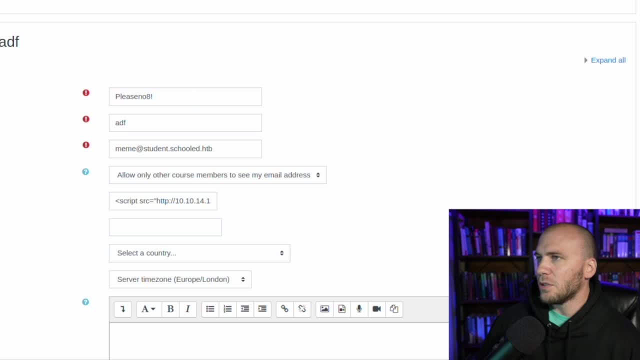 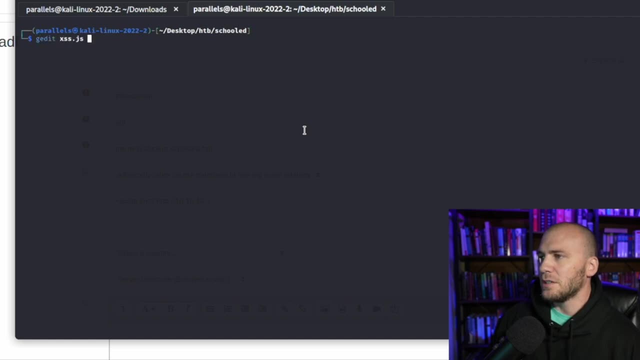 if it doesn't work, i can go and fix that. so now what we'll do is go to our cali machine over here, and we have used the python server in the past. but the first thing we need to do is g edit, and i've actually already written out the script here for us, and we have a document dot write. this is: 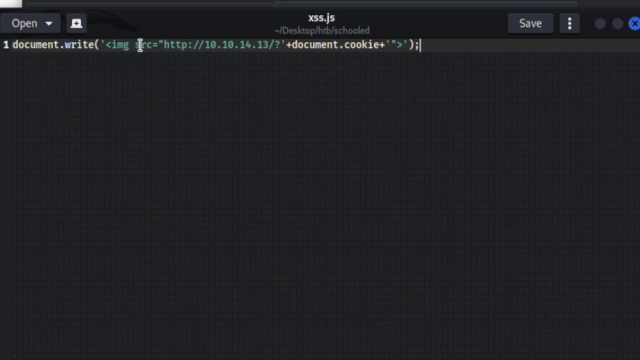 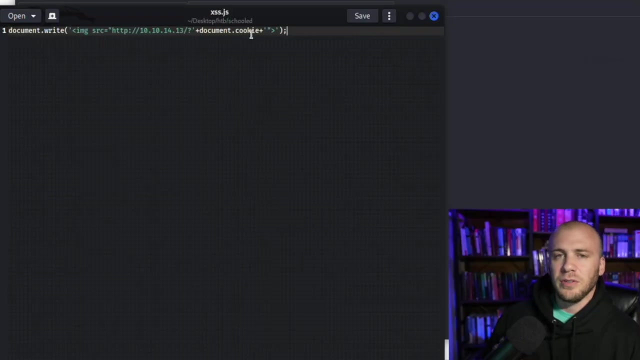 just javascript. so we're wanting the javascript to write something for us. it's going to use our ip address right here and then it's going to send the cookie to us. so if you want to grab a bunch of different cross-site scripting payloads, it's really simple. you can just type in cross-site. 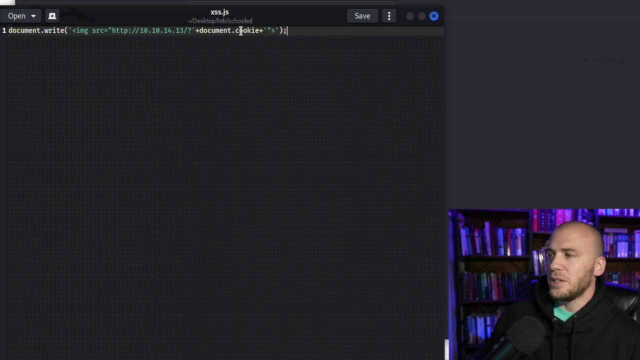 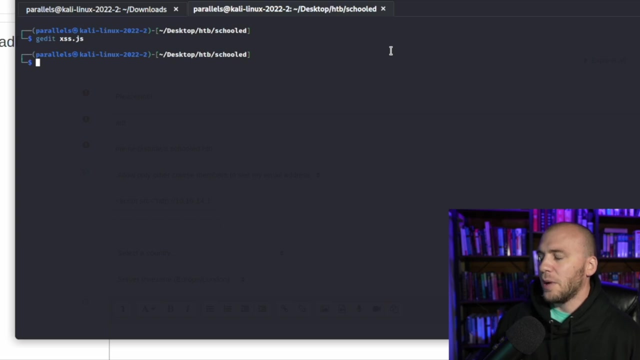 scripting payload into google and then just search through github pages and there's going to be hundreds, maybe even thousands of different cross-site scripting payloads that you can try to see if any of them will work, if you don't know javascript, and so we'll save this. and now what's going to happen is we're going to host this up with a python server. 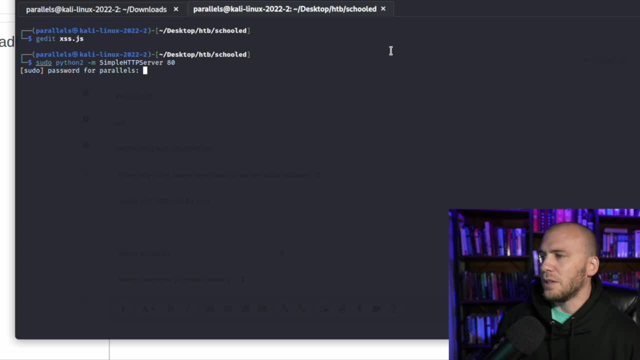 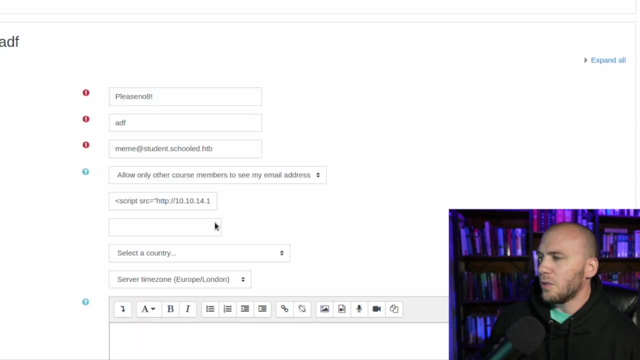 so we'll type in sudo, python 2 and then we'll run this simple server right here and now we have it listening right here. so this file is now going to be accessible. so what's happening is this is going to execute, the server is going to reach us and it's going to send us a message that says: 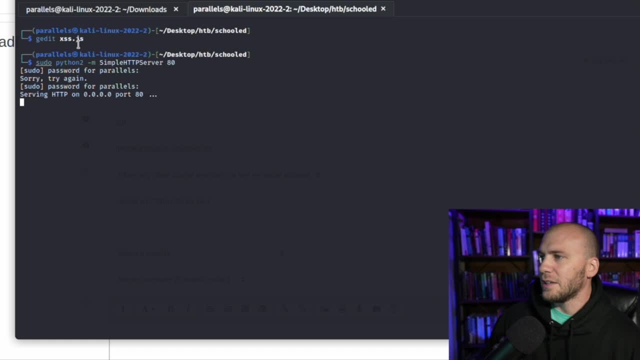 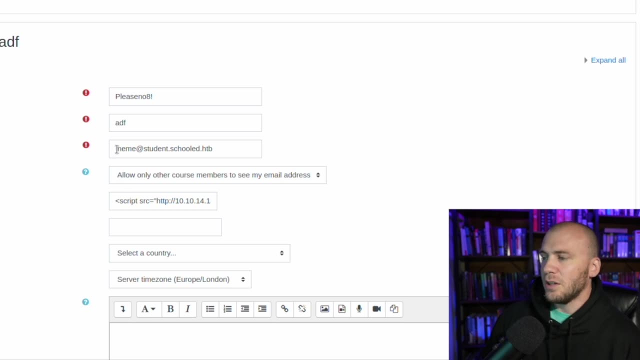 welcome to our python server right over here. that's listening and it's going to grab this file, it's going to execute the javascript and then it's going to return us the cookie once it's executed on this server. so what would typically happen is you would put this cross-site scripting onto a 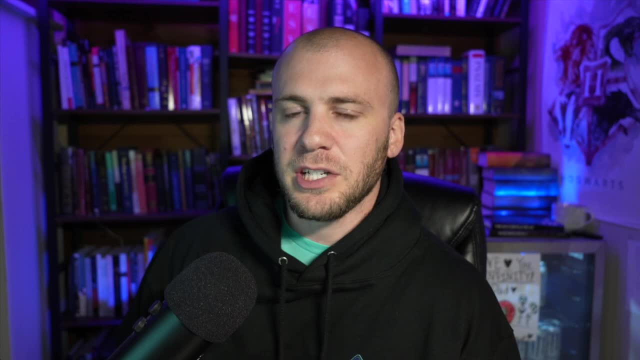 server and then you'd have to wait for somebody to come to this page and execute the payload or view the profile in this specific case, and then you would steal their cookie and you could potentially use that cookie to hijack their session. so we can come down here and we'll.